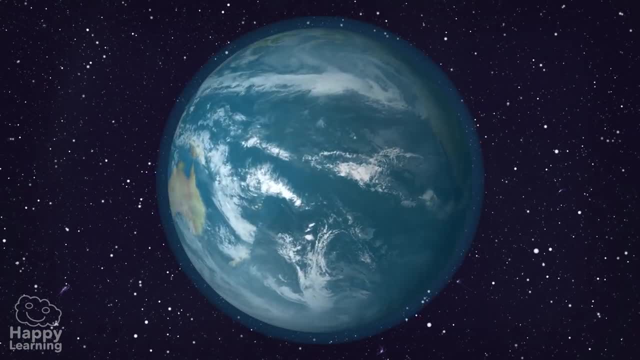 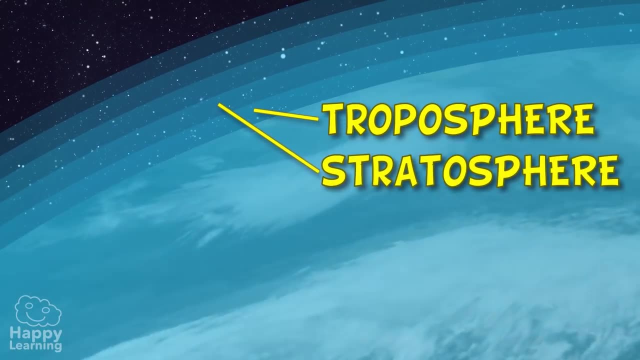 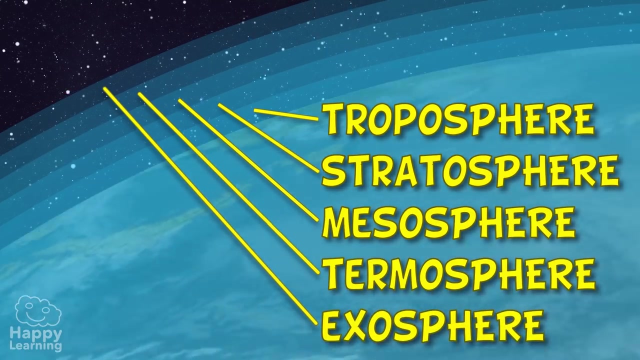 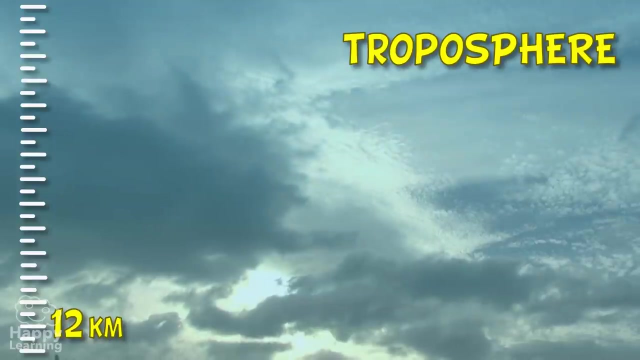 Because of those differences, we divide the atmosphere in five layers called the troposphere, stratosphere, mesosphere, thermosphere and exosphere. We are going to know more about each one of them. The troposphere is an interior layer, the closest one to the Earth's surface. 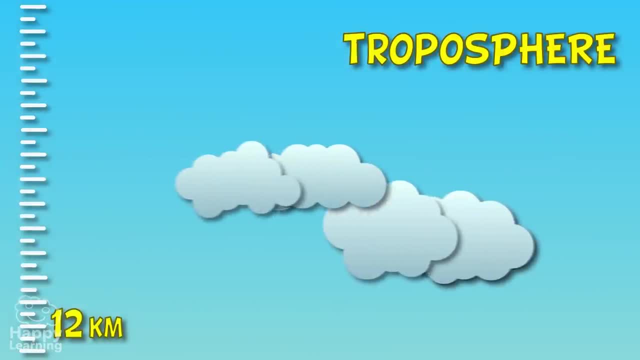 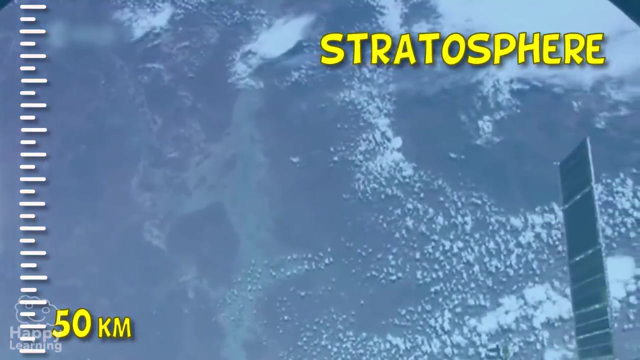 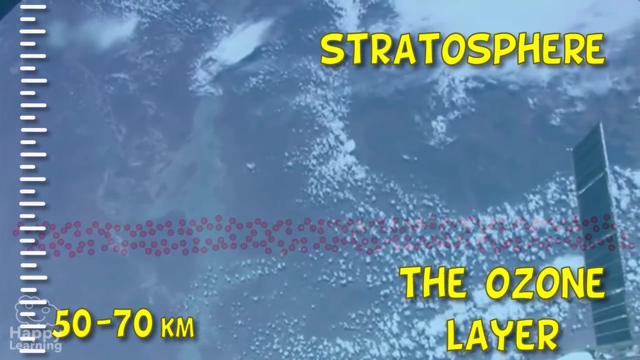 It reaches 12 kilometres in height and within it is where the phenomenon we call the weather happens- the climate. The stratosphere reaches an average height of 50 kilometres, although in some points it reaches 70.. Inside the stratosphere we can find the ozone layer, which is essential for life because it filters ultraviolet light coming from the sun. 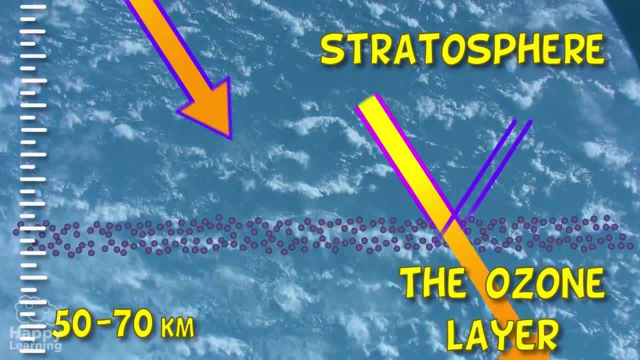 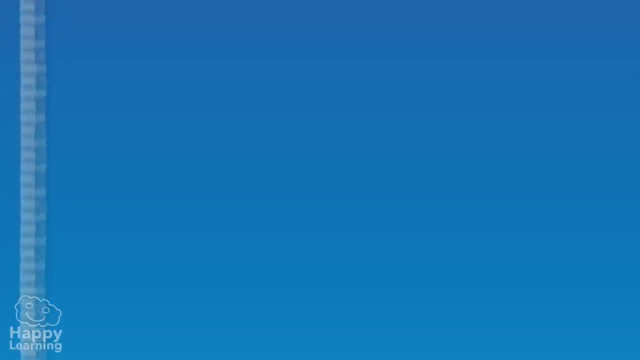 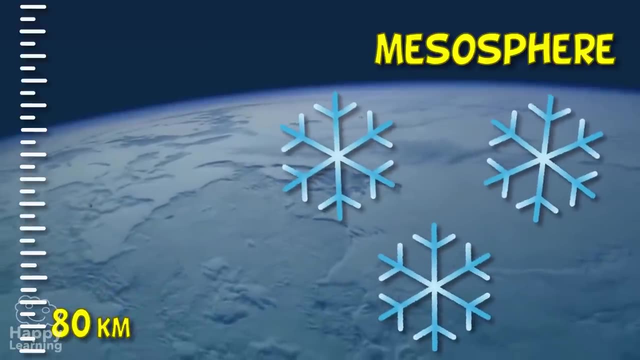 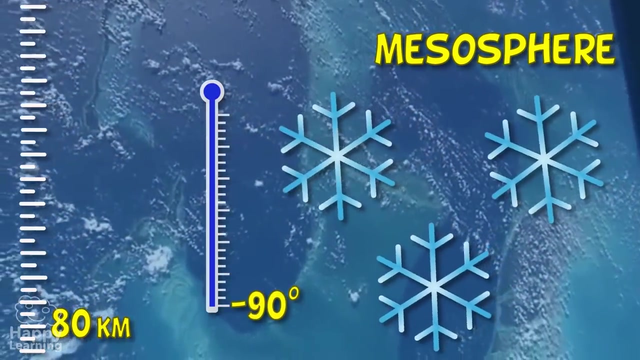 If it didn't exist, these rays would end life on our planet. The mesosphere is situated between 50 and 80 kilometres over the Earth's surface. It's the coldest layer in the atmosphere. It can reach less than 90 degrees below zero. It's so cold. 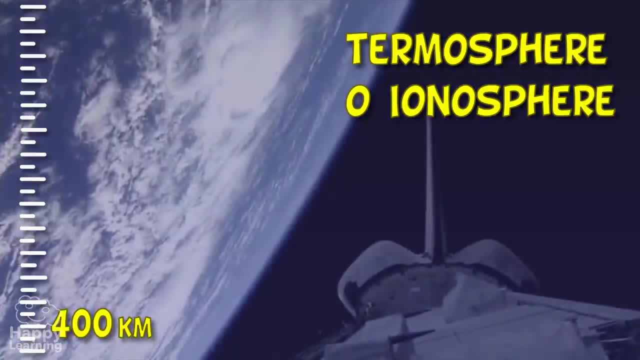 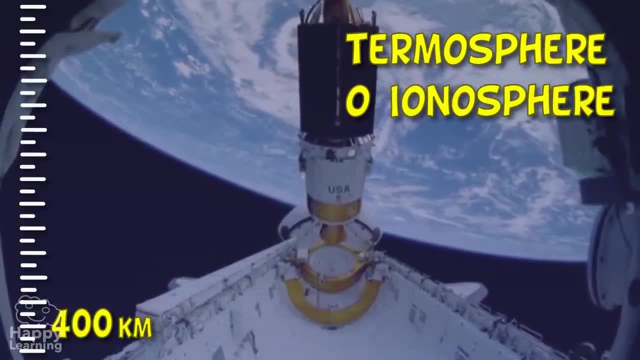 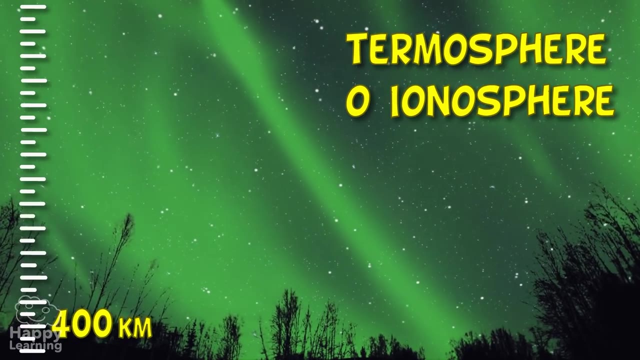 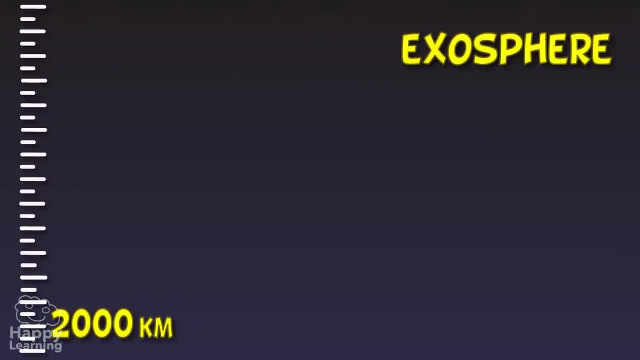 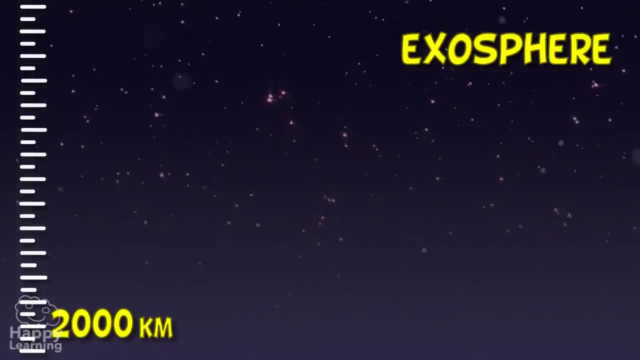 The thermosphere, also called ionosphere, reaches 400 kilometres. Within it, space shuttles travel around the Earth, and it's also where the mysterious northern lights take place. They're beautiful, aren't they? The exosphere is the last layer in the atmosphere and is situated between 400 and 2,000 kilometres. 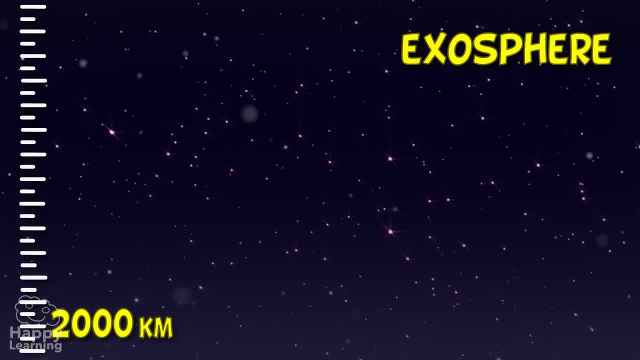 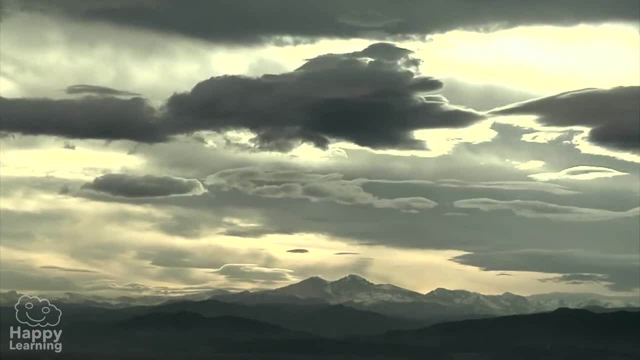 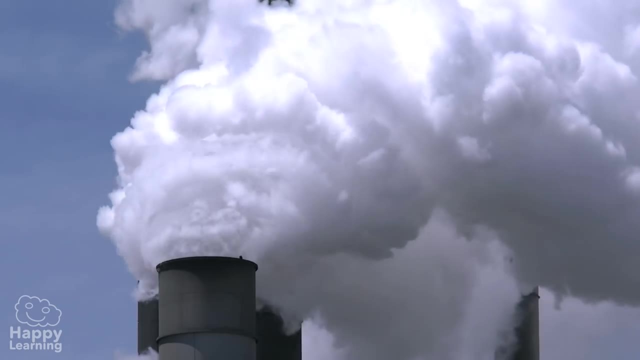 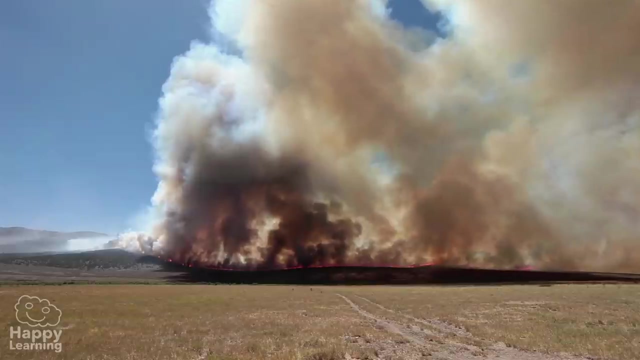 After this, there are no more gases, only the emptiness of space. Now we know all about the atmosphere and its layers, but we can't say goodbye without talking about pollution. Human activity releases many gases that contaminate our atmosphere: Smoke from factories, cars. lots of the daily activities we do are creating changes in the atmosphere's composition.